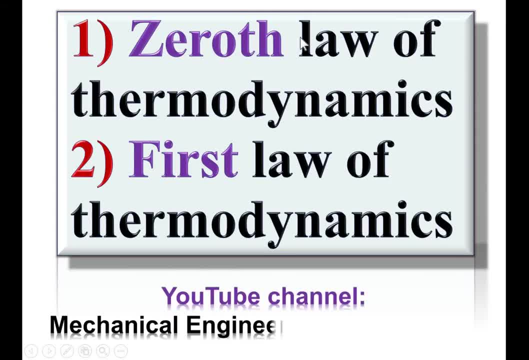 Today we are going to discuss about two topics: First, zeroth lobe thermodynamics and second, first lobe thermodynamics. So welcome to my YouTube channel, Mechanical Engineering Management. So let's start from the zeroth lobe thermodynamics. 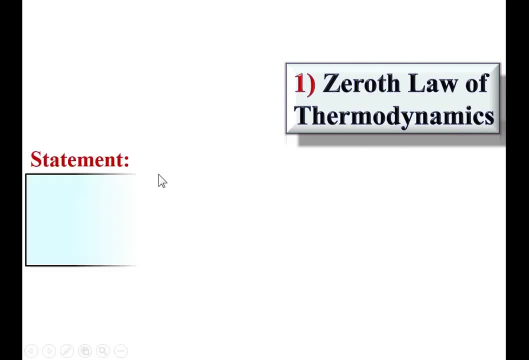 So first the statement of the zeroth lobe, thermodynamics, If two bodies, A and B, are in thermal equilibrium with third body C. So up to here this is the condition: There are the two bodies A and B, and both are in thermal equilibrium with the body C. 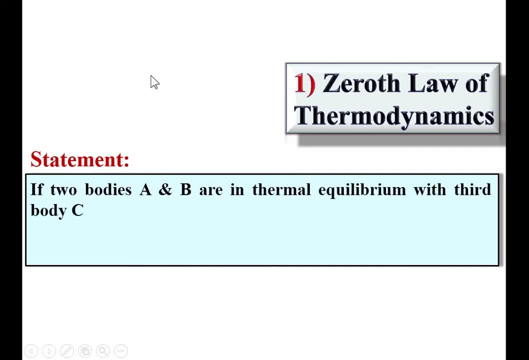 So try to understand this condition with the help of the figure first. So let's say this is the body A and this is the body B. According to the statement, if the body A is in thermal equilibrium with the third body C, then the body B is in thermal equilibrium with the third body C. 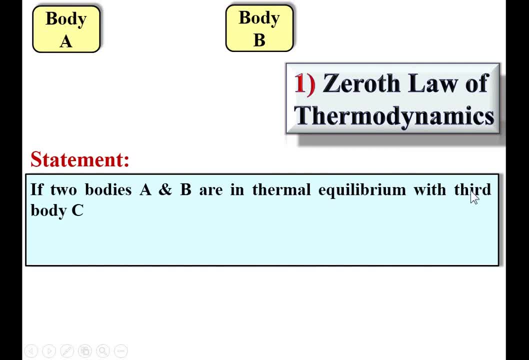 If the two bodies, A and B, are in thermal equilibrium with the third body C. So let's say over here: this is the third body C and both A and B are in thermal equilibrium with the body C. So I can say this: both body are in thermal equilibrium with the body C. 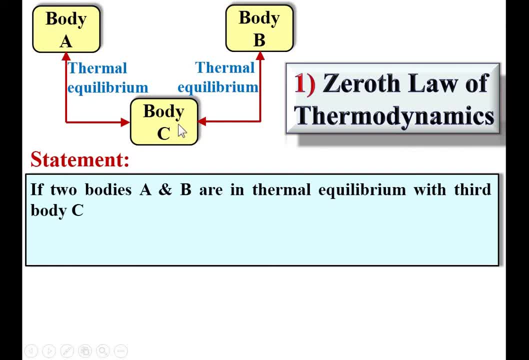 Thermal equilibrium, that means the temperature is same of both body, then this is called in thermal equilibrium. So once again, look at this statement: If two bodies, A and B, are in thermal equilibrium with the third body, C, that we have shown over here in this figure. Now next then. 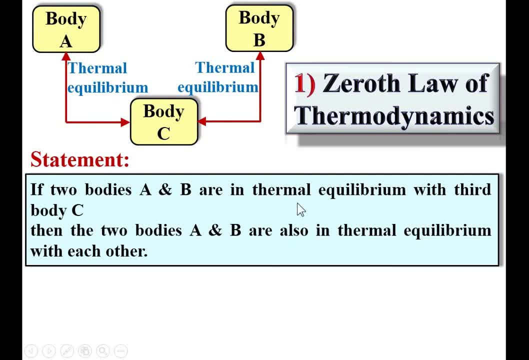 the two bodies, A and B, are also in thermal equilibrium with each other. So I can show over here in this figure that both body A and B are also in thermal equilibrium. The principle of temperature measurement is based on zeroth law of thermodynamics. Now why it is called zeroth? 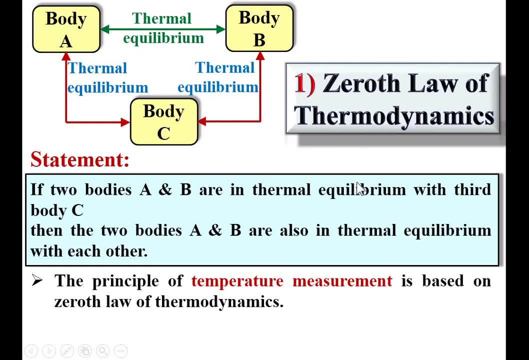 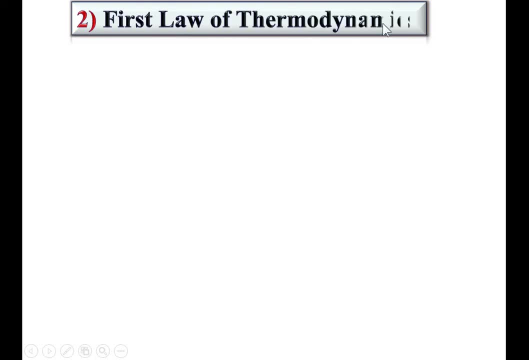 law of thermodynamics, Can you imagine? So this is the answer. This law was stated after first law of thermodynamics, Hence it is called as zeroth law of thermodynamics. Now the next one, first law of thermodynamics. So focus over here carefully, because of it is a little bit difficult. 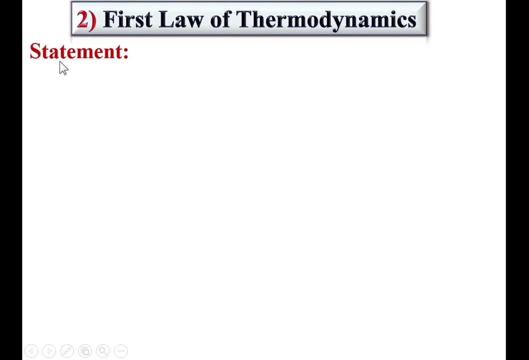 Compare to the zeroth law of thermodynamics. First, start with the statement: Energy can neither be created nor be destroyed, but it can be converted from one form to the another form. So it is basically the law of conservation of energy. So it is very simple. 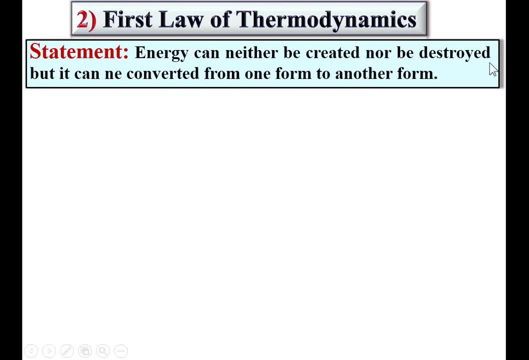 energy can neither be created nor be destroyed, but it can be converted from one form to another form. Thus it is a statement of law of conservation of energy When a system undergoes change of state, and that we have discussed in the earlier video of basic terminology like state path cycle process, So you can refer it. 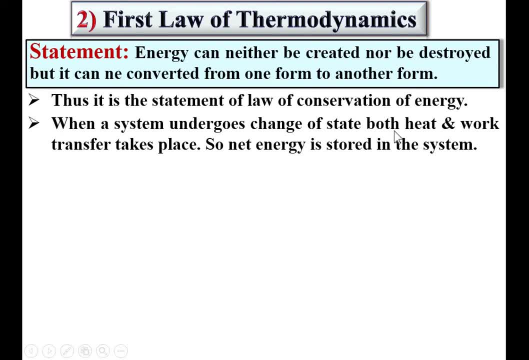 So when a system undergoes change of state, both heat and work transfer take place. So the net energy is stored in the system. So I can say the net energy stored in the system is equal to heat supplied minus work done. So whatever it may be the difference of the heat supplied and work done, 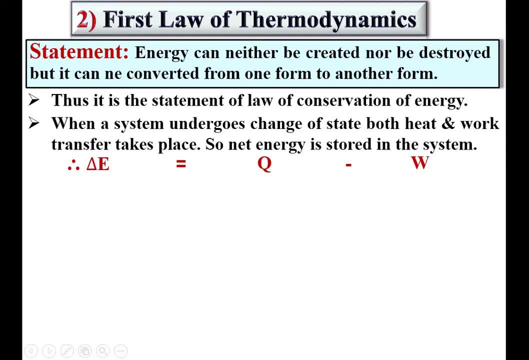 that will be stored in the system, that is called as the stored energy and that is represented by delta E. So I can say delta E is the net energy stored, is equal to Q, that means heat transferred to the system, minus W, that is the work transferred. and as you know that the stored energy is the 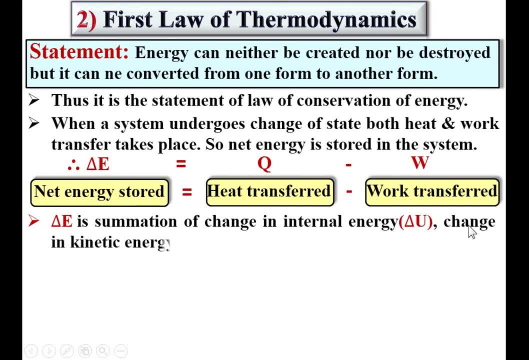 summation of the change in internal energy delta U, change in kinetic energy delta Ke and change in potential energy delta Pe. For a closed system, mass is fixed, So there is no elevation and movement. No elevation- that means there is no change in potential energy. No movement- that means no. 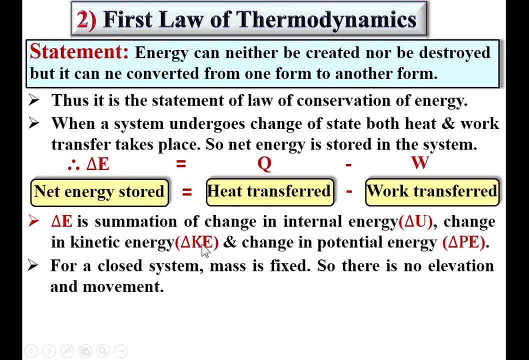 velocity, that means change in kinetic energy is zero. So for a particular closed system I can say: delta E is equal to delta U. only because of this both term will be zero. So I can say: for a closed system change in potential energy is equal to zero and change in kinetic energy is.